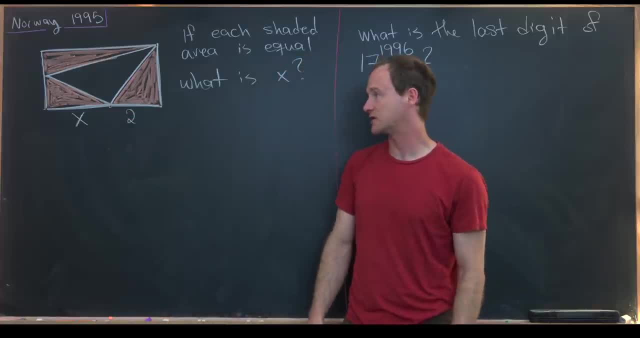 vertex is equal to two And our goal is to find the measurement of x. So let's get to it. And I should point out that when we're talking about the areas of these triangles, we're in fact going to talk about twice the areas of these triangles, just so that we don't. 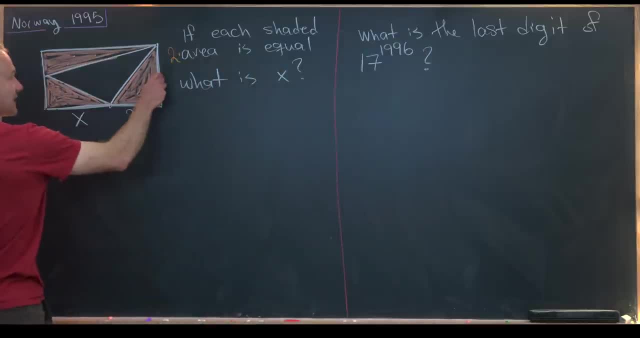 have to divide by the two. So we'll start by saying that the height of this rectangle is y, which means that twice the area of all of these triangles is 2y. Okay, But that means we can find this line segment length here, In other words, the height of this kind of bottom left triangle. 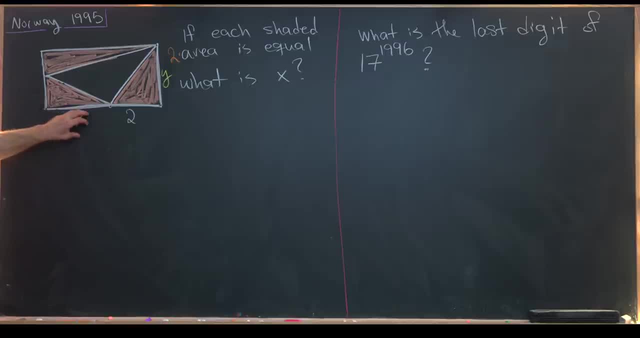 We know that this number right here times x must be equal to 2y. That means that this length right here must be 2y over x. Notice: 2y over x times x is 2y. 2 times y is also 2y. 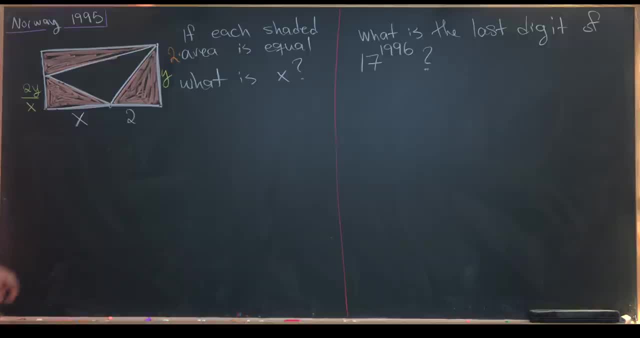 And then next we know this entire line segment has length y, which means this entire line segment has length y, So that all of this bit that's left over is y minus 2y over x. So now notice, if we add this line segment and this line segment, we get the length y. 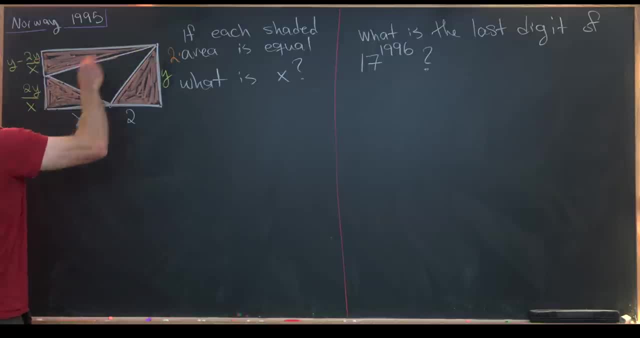 which is what we want. Finally, we can fill in the length of the rectangle as x plus 2.. Now we can set up an equation. So, given the fact that all of these three triangles have the same area, we know the area of this triangle is equal to the area of this triangle. But 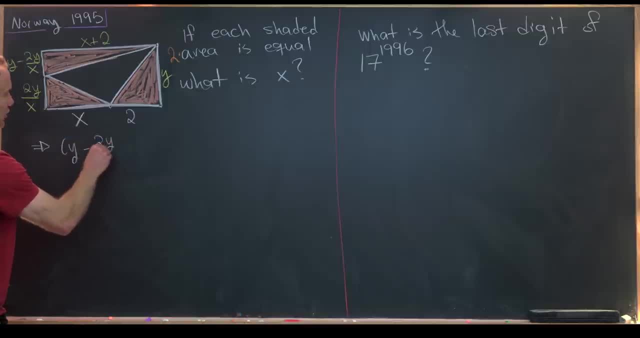 that tells us that y minus 2y over x times x plus 2 must be equal to 2 times y. Notice, we've got this extra y term here, but we could divide that extra y term out and cancel it. on the other side of the equation, That's allowed, because y is not 0, given that we do not have a, 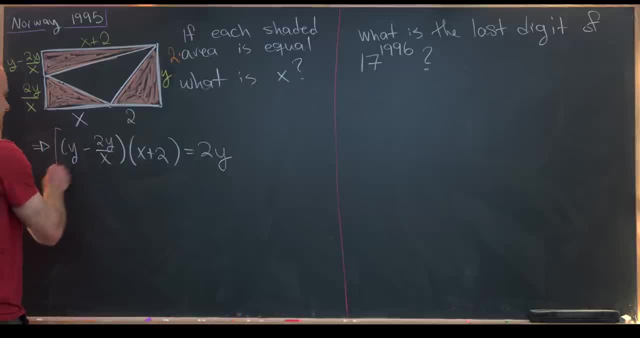 degenerate rectangle here. So just to reiterate, I'm going to take both sides of this equation and multiply by 1 over y. So that's going to have the effect of canceling this down to 1, canceling this and canceling this. 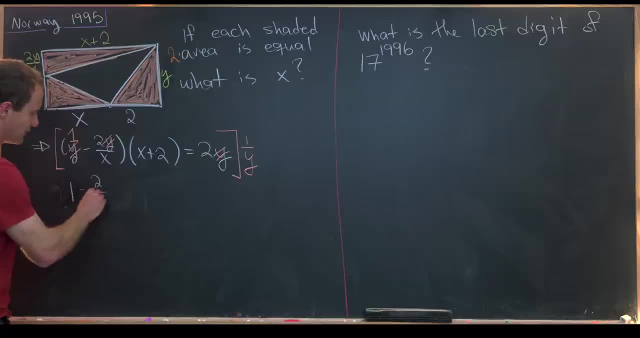 That leaves us with 1 minus 2 over x times x plus 2 equals 2.. So maybe just to make this look a little nicer, I'll multiply both sides of this equation by x. Now we have x minus 2 times x plus 2 equals 2x. Multiplying out the left-hand side and moving this: 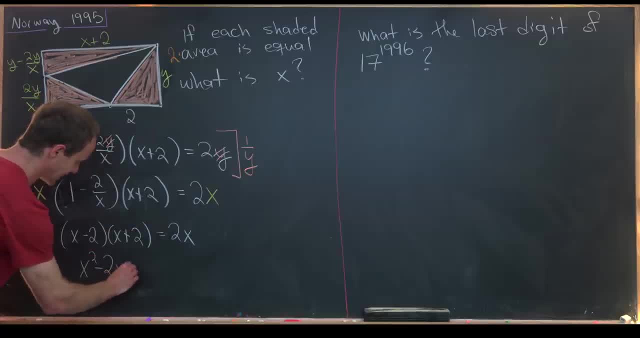 2x over leaves us with x squared minus 2x minus 4 equals 2x. Now we can attack this by using the quadratic formula to solve for x. So doing that, we'll see that x equals 2 plus minus the square root of- well, it's negative 2 squared minus 4, times negative 4,. 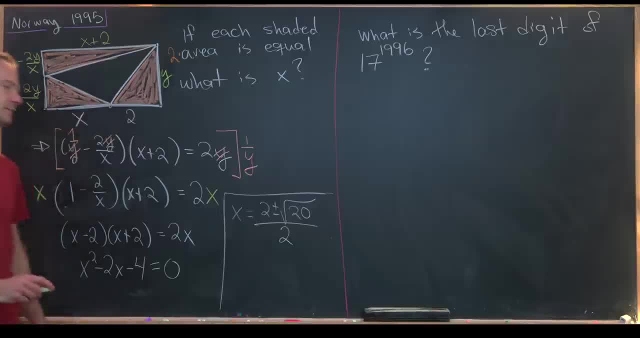 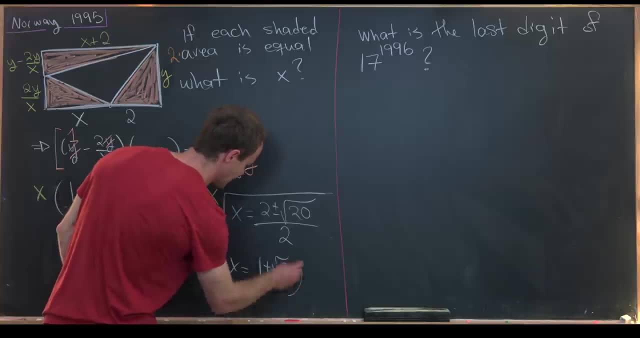 so that's going to be 20 over 2.. Then, doing some simplification, we see that our x value must be 1 plus root 5. And that would be minus sign because that would correspond to having a negative line segment length here. 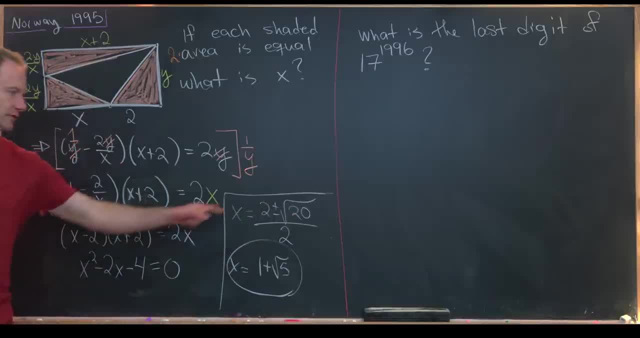 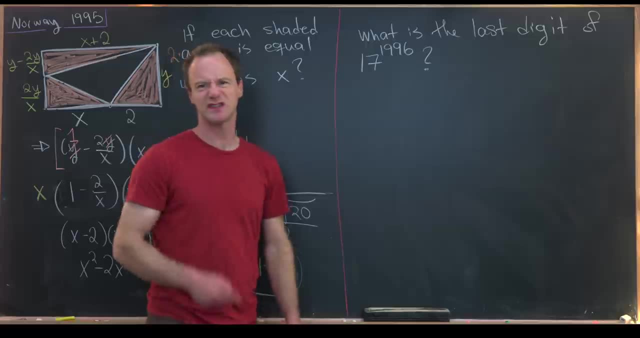 And we can also factor a 4 and take the square root out of this square root, leaving us with this 1 plus root 5.. Ok, so now let's look at our next problem, which is like a nice little number theory trick problem. 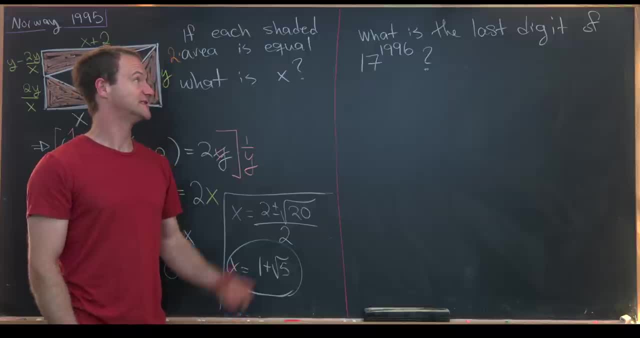 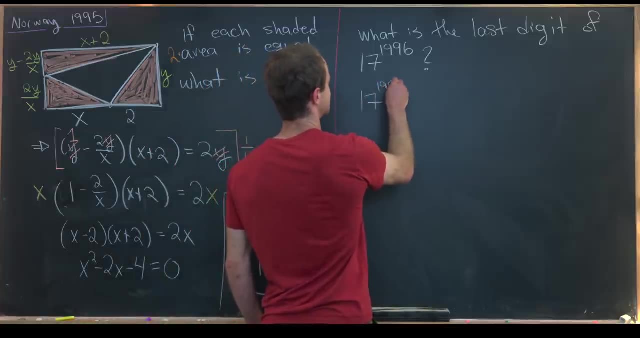 So we want to find the last digit of 17 to the 19, 96.. So, put in other words, we want to calculate 17 to the 19, 96, mod 10.. So recall that reducing mod 10 will give us the last. 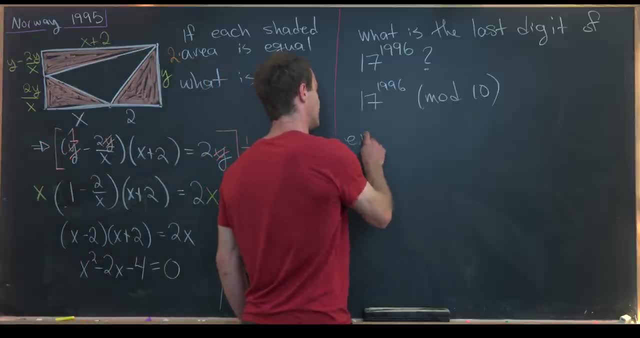 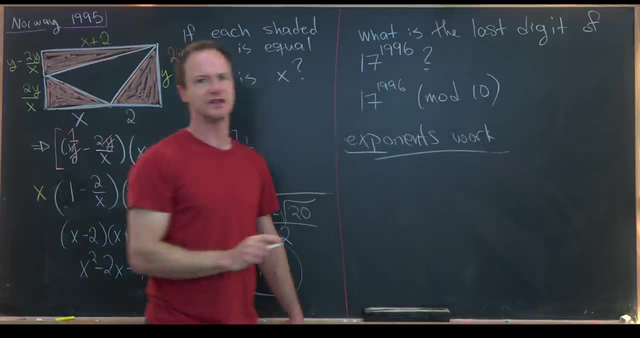 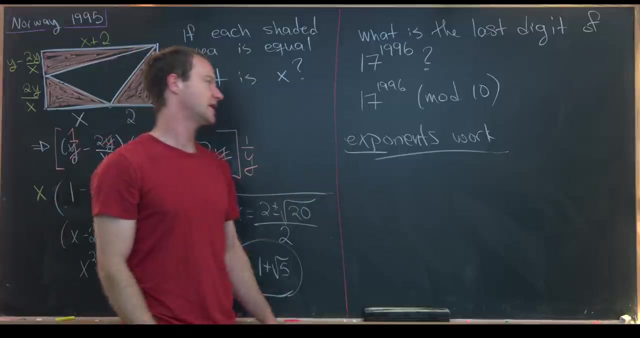 digit. So we want to remember that if we're reducing mod n, then exponents will work, mod phi of n, which is Euler's phi function, which counts the number of numbers that are relatively prime less to n. So here we want to notice that the exponents work. 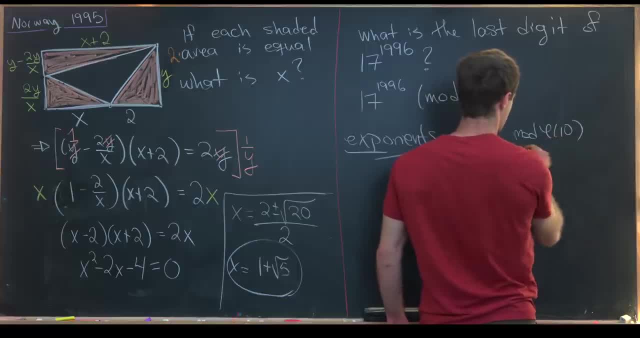 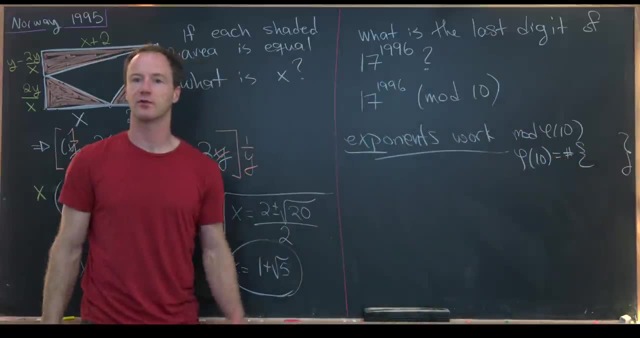 Mod phi, Phi of 10.. But we might want to calculate phi of 10.. So that's going to be the number of elements in this set from 1 to 10 that are relatively prime to 10.. It's easy to make a list of that, though.